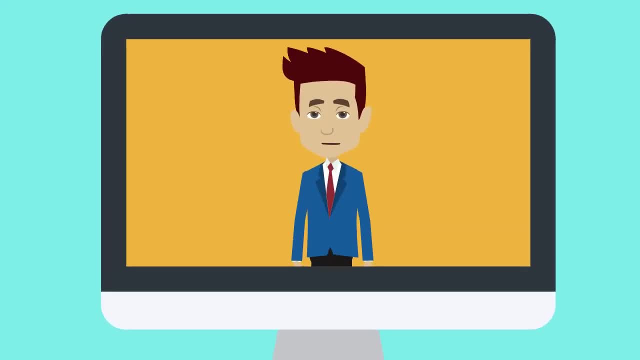 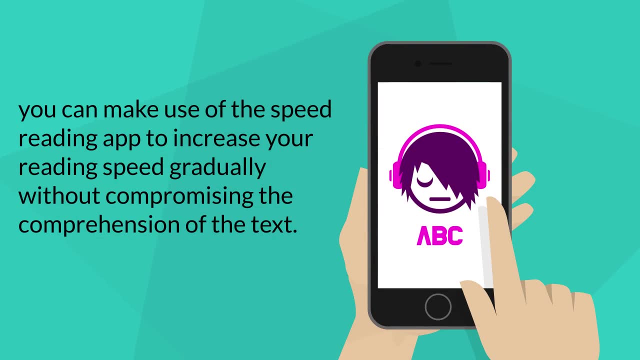 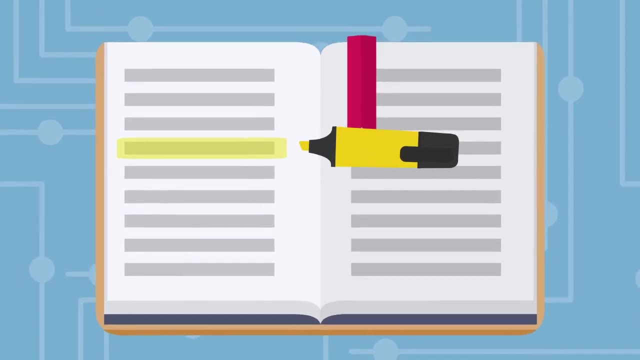 of the first sentence carefully. As discussed in the earlier video, you can make use of the speed reading app to increase your reading speed gradually without compromising the comprehension of the text. The next technique I would suggest is to highlight any line you find important while reading through the text, so that you don't miss that key point in the text. 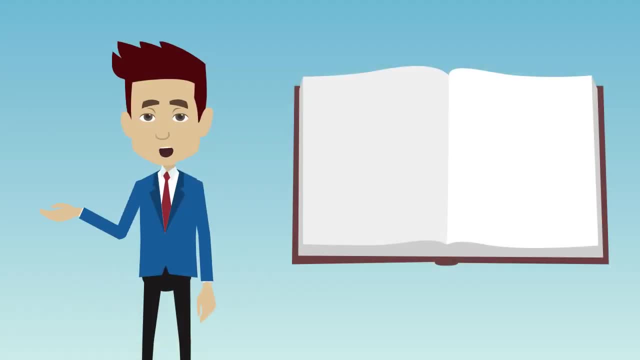 The natural way to go about reading a text is to garner the entire theme of the text by reading the first and last paragraph of the text, Then proceed further by reading the initial sentence of each paragraph carefully to get an idea of the entire paragraph, and then gradually, 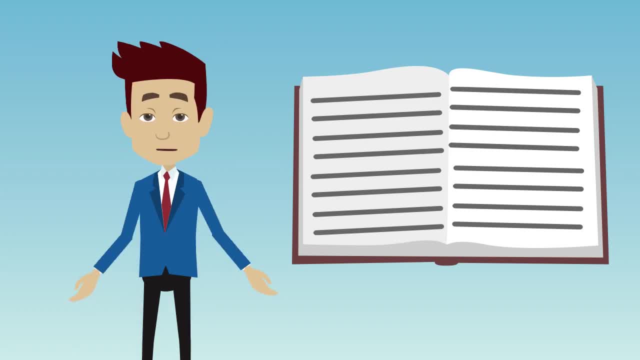 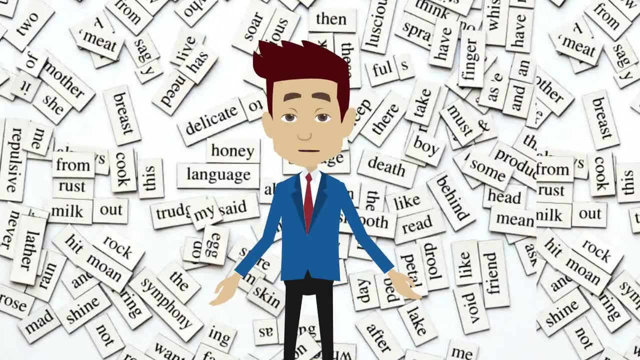 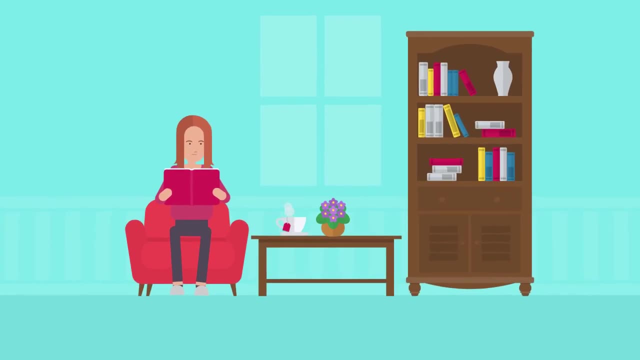 increasing the reading speed for the remaining text of the paragraph. Now we will discuss about answering reading comprehension questions in your exam. Please remember that better knowledge of vocabulary helps you understand the text effectively and reading it faster. So please focus on improving your vocabulary. 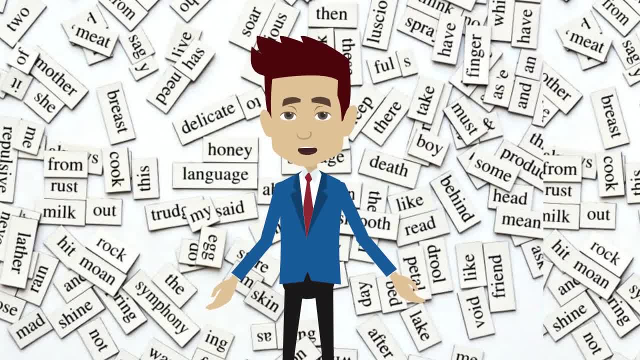 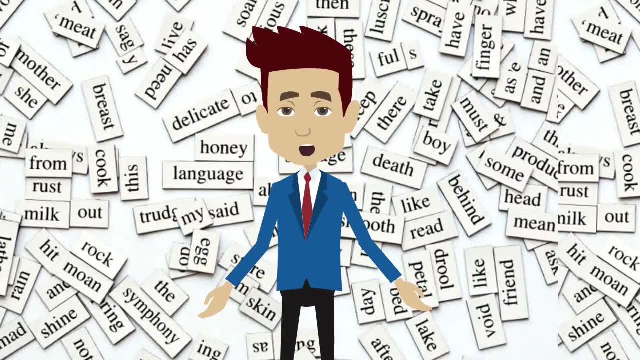 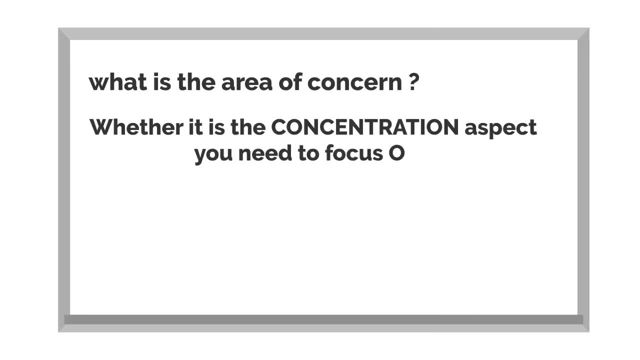 I've already discussed ways to improve your vocabulary in previous videos. Also, continuously evaluate yourself after practicing comprehension passage, identifying the areas you need to improve on. For example, what is the area of concern? Whether it is the concentration aspect you need to focus on, whether it's the vocabulary. 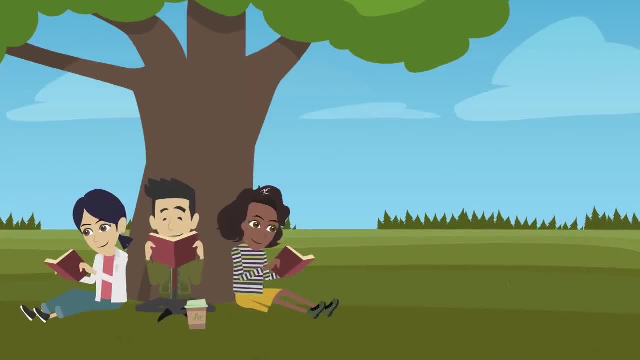 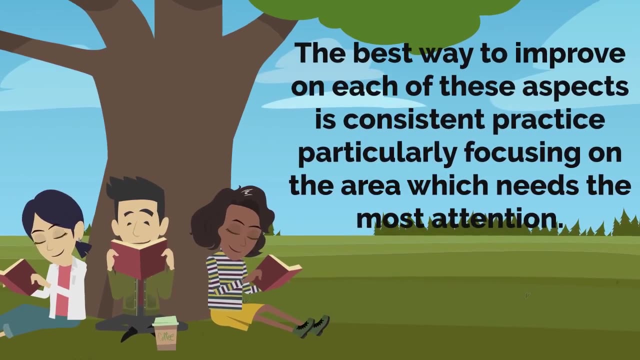 whether it's the reading speed you need to work on. the best way to improve on each of these aspects is consistent practice, particularly focusing on the area which needs the most attention. Now let us discuss about some useful things to be kept in mind while solving a reading. 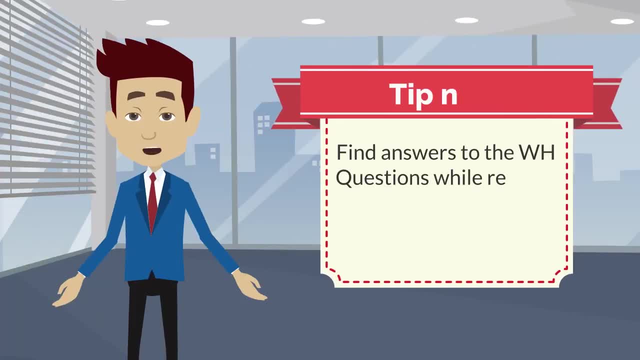 comprehension passage. Tip number one: Find answers to the WH questions while reading a passage, such as who, what, where, when and why. Tip number two: Try to visualize the passage to remember and retain it. Tip number three: Organize the key information. 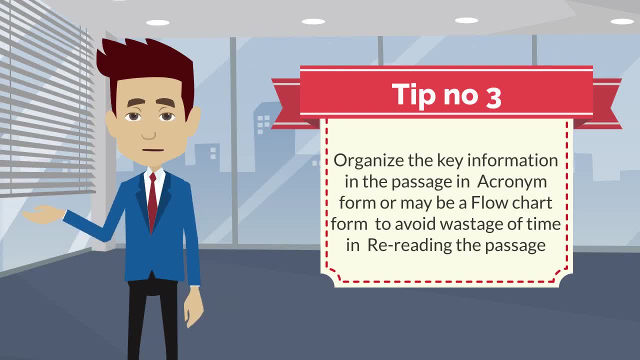 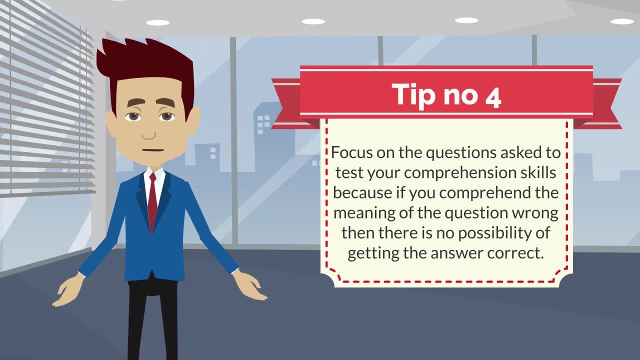 in the passage in acronym form or maybe a flow chart form, to avoid wastage of time rereading the passage. tip number four: focus on the questions asked to test your comprehension skills, because if you comprehend the meaning of the question wrong then there is no possibility of getting the answer correct. tip number: 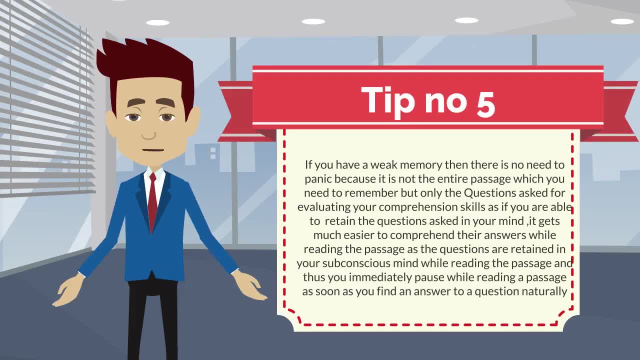 five, if you have a weak memory, then there is no need to panic, because it is not the entire passage which you need to remember, but only the questions asked for evaluating your comprehension skills, as if you are able to retain the questions asked in your mind, it gets easier to comprehend their answers while